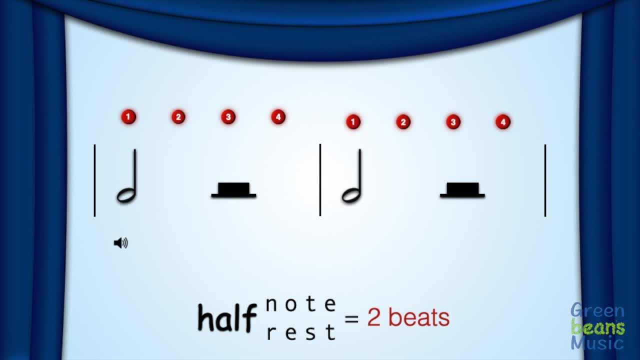 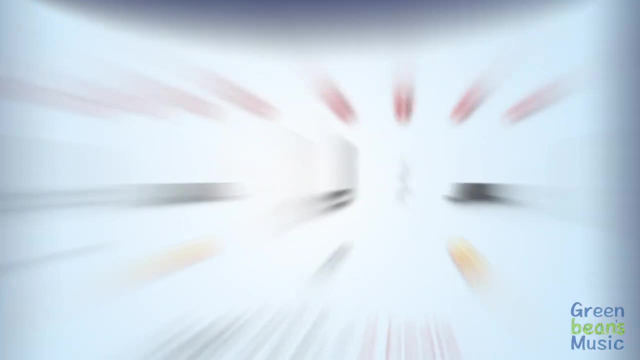 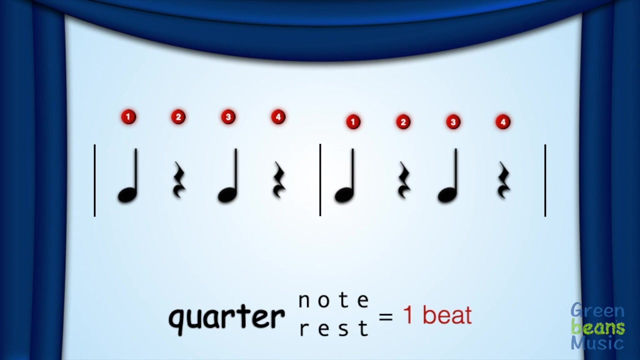 Okay, your turn. One more time, One more time. Okay, now we have quarter notes on beats one and three and quarter rests on beats two and four. Let's clap this One more time. Good, Now let's reverse the order. 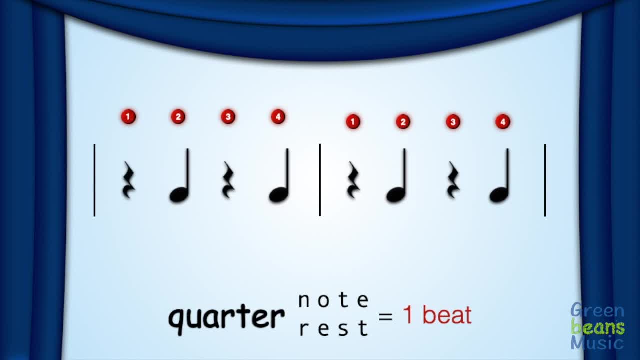 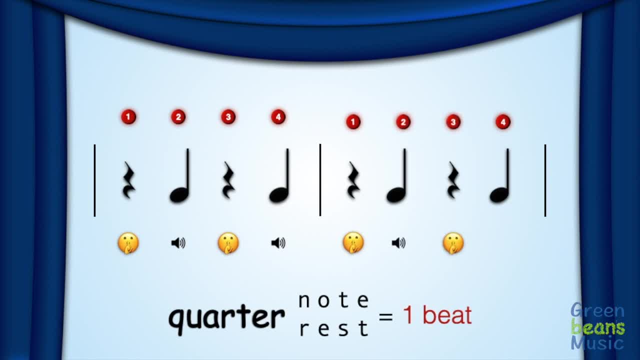 Again, Again, Again, Again, Again. Now let's do some eighth notes and eighth rests. Again, Again, Again, Again. And now let's reverse the order. And now let's reverse the order. And now let's reverse the order. 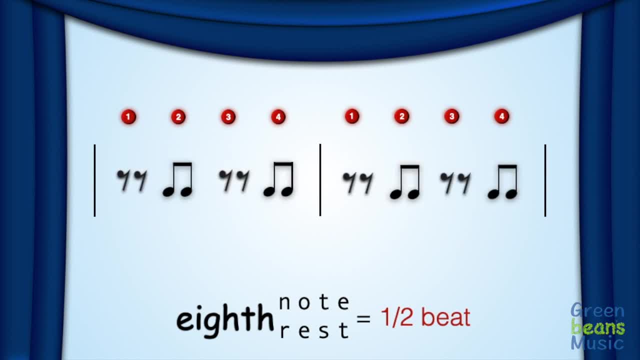 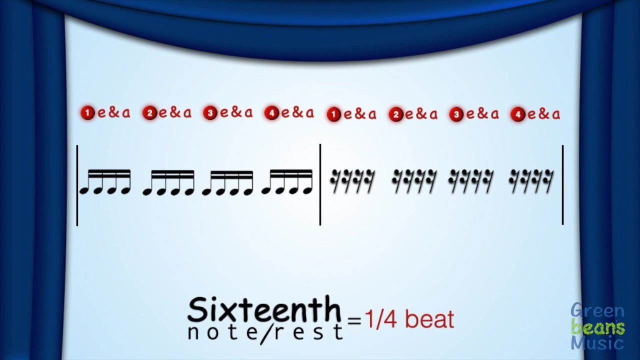 Okay, and now we rest on beats 1 and 3, and we have 8th notes on beats 2 and 4.. One more time, One more time. 16th notes and rests. For our example, we're using a full measure of 16th rests, but we could easily replace them with one whole rest and accomplish the same goal of 4 beats of silence.